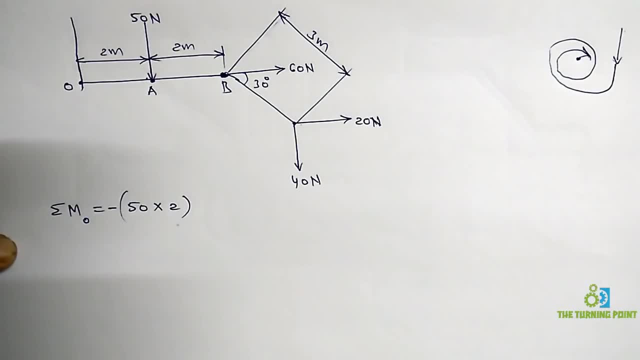 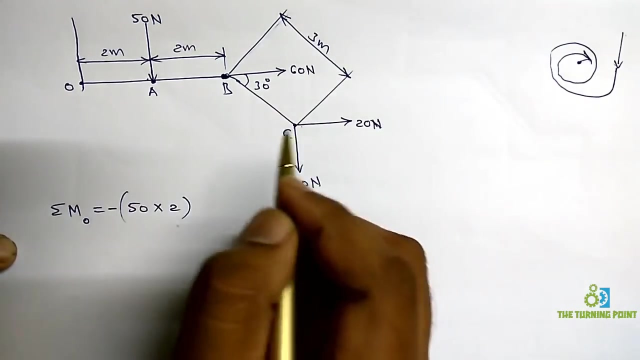 because of that force will be zero. Moment because of that force will be zero. So no need to calculate moment for that. and the remaining forces are 20 newton and 40 newton. Now we have to consider perpendicular distance for those two. So I know here BC distance is given as 3m. 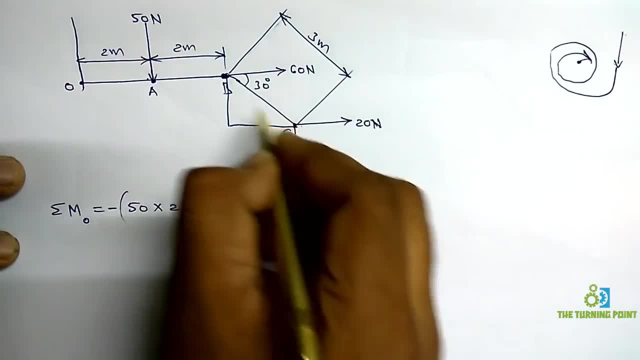 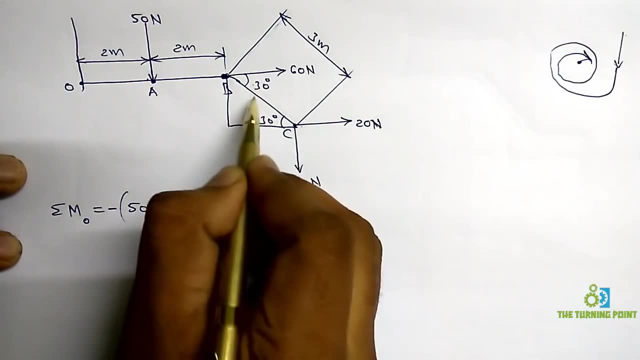 Right, So I can find perpendicular distance between those. So here, if this is 30°, this is going to be 30°, Right? So here, this is in the form of a right angle triangle. So here, this is 3m, This is 30.. So then it will become: 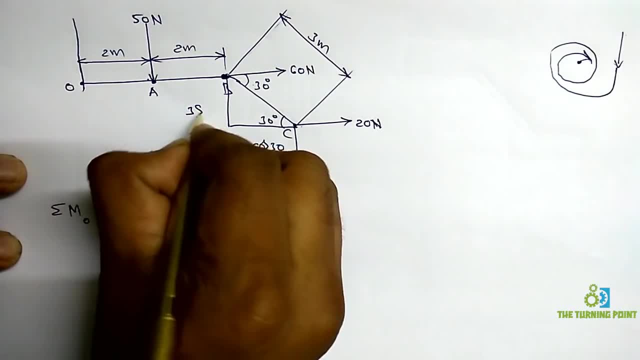 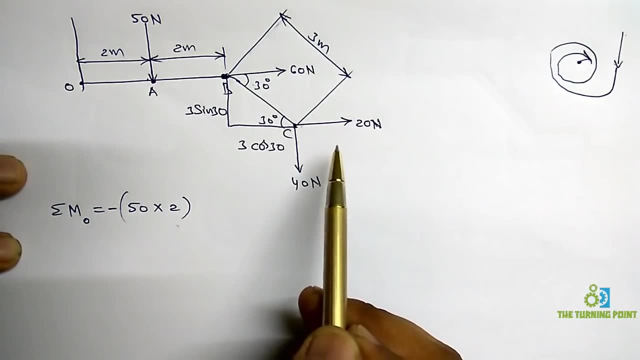 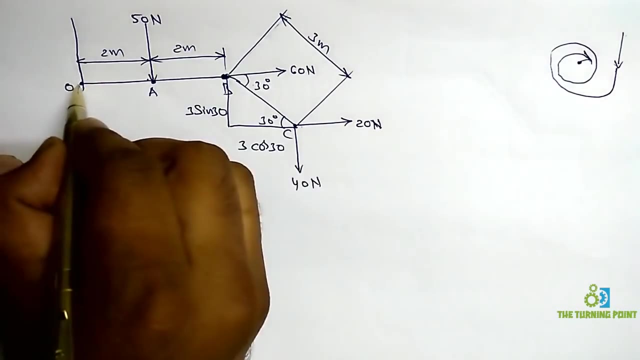 3 cos 30. It will become 3 sin 30.. Right moment, because of 16 newton force, is zero. next we will consider 20 newton force 20 into perpendicular distance. draw a line passing through moment center parallel to consider: 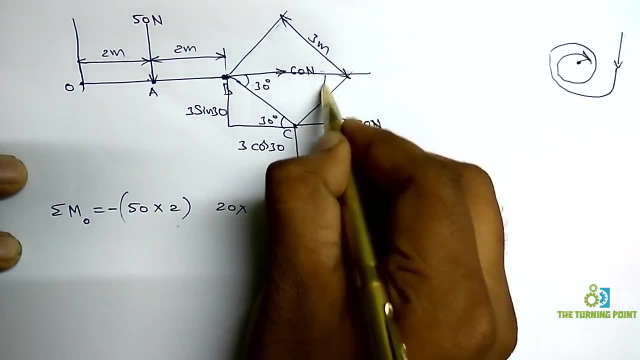 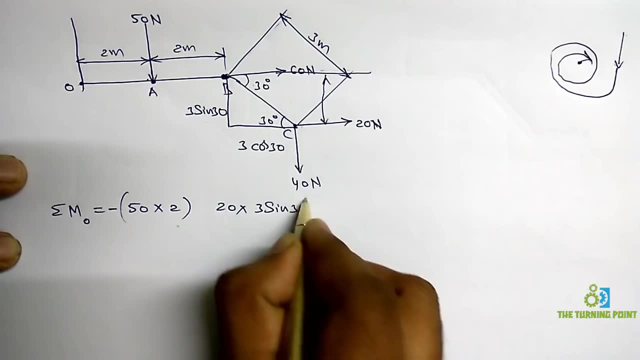 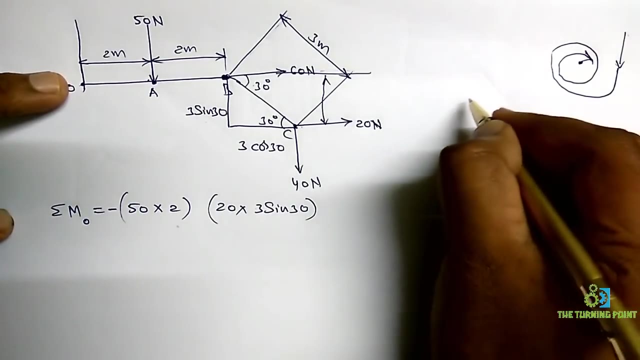 force. so then a line will appear like this. so it will be like this. so then this is the perpendicular distance. thus, distance is nothing but 3 sin 30, right, 3 sin 30. so if you want to find whether it is clockwise or anti-clockwise, so moment center is here, o is here, and 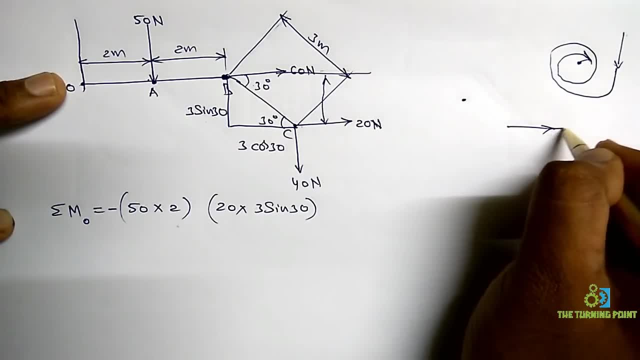 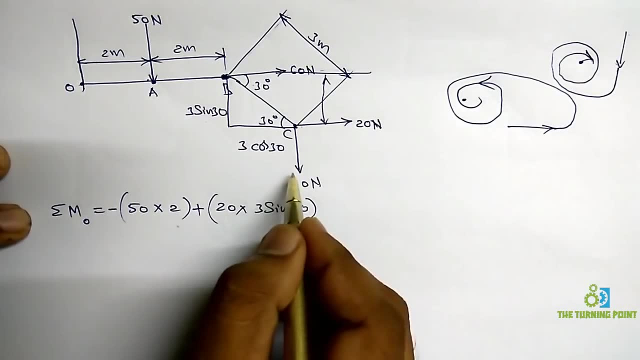 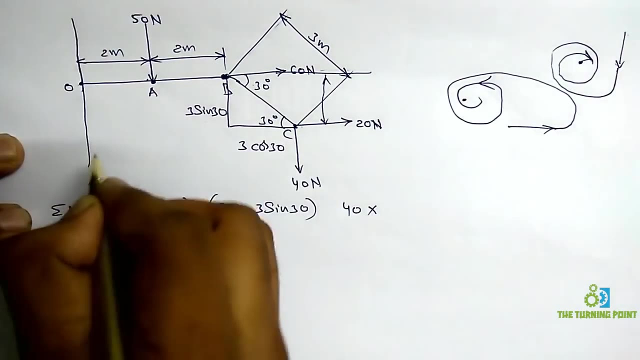 force is here. 20 newton force is here. in the direction of force, encircle the moment center how i am doing here. anti-clockwise means positive. next, 40 newton force, 40 into perpendicular distance. draw a line passing through moment center, parallel to consider. 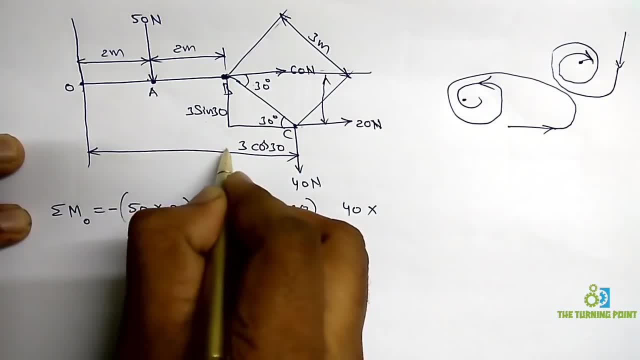 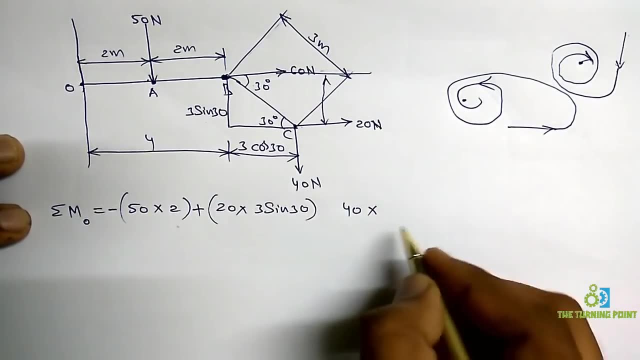 force. so then this is the perpendicular distance, right, it is nothing but. so 2 plus 2, that is 4. 4 plus 3 cos theta. right? so so that is 4 plus 4 plus 3 cos theta. right? so so that is 4 plus 3 cos theta, right, so so that is 4 plus. 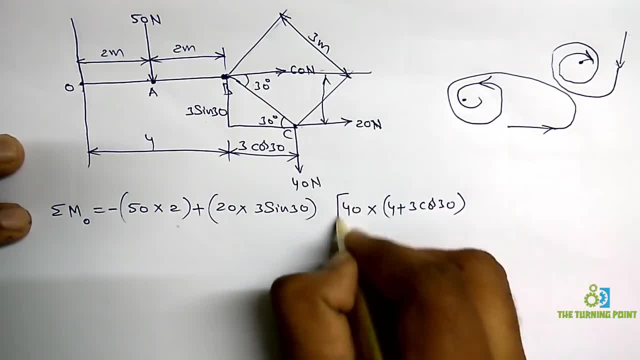 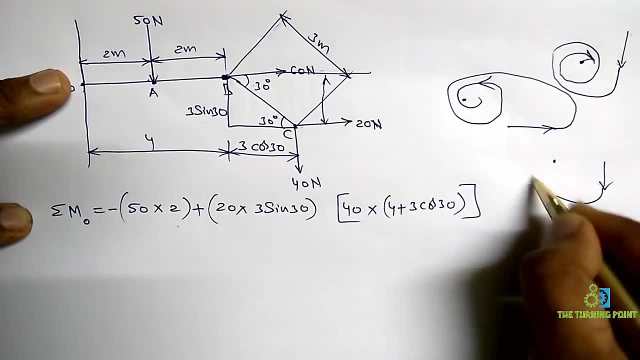 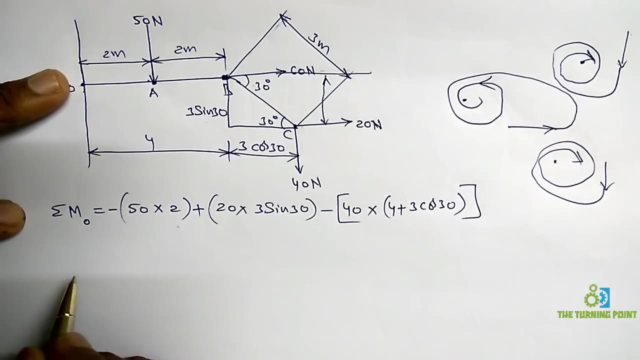 3 cos theta. so to find whether it is clockwise or anti-clockwise moment center here. and application of force is here in the direction of force encircle the moment center. so it is happening in clockwise sense. so clockwise means negative. so if you simplify this one you will get the 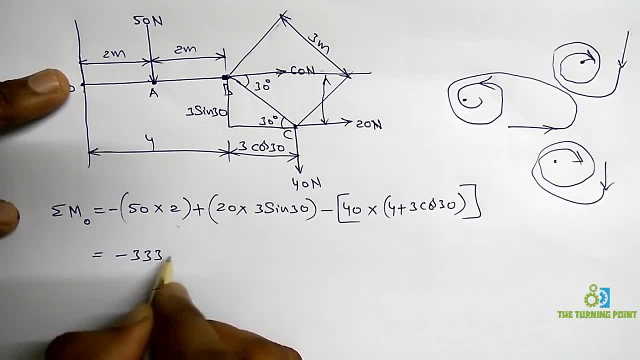 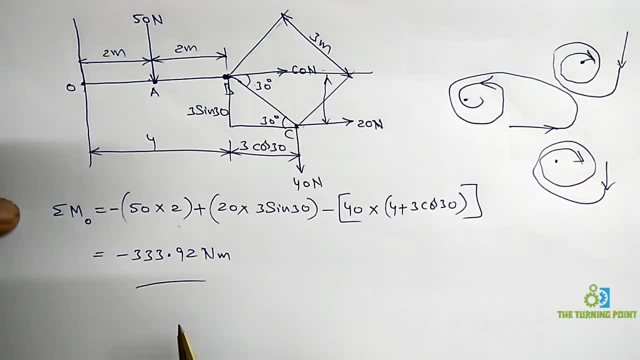 value for moment about o, so you will get around minus 333.92 newton meter. hope you like this video. click on like button and don't forget to subscribe. thank you for watching.